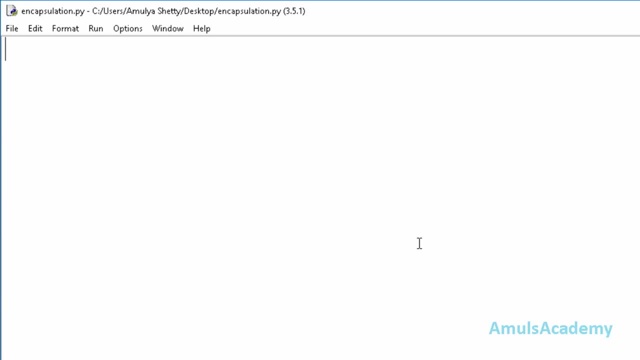 to prevent that by being modified. So we use encapsulation and there are two types of access specifiers: one is private and another is public. Till now in the example, we use public methods and public variables. That means we can access them outside the class also. That is this. 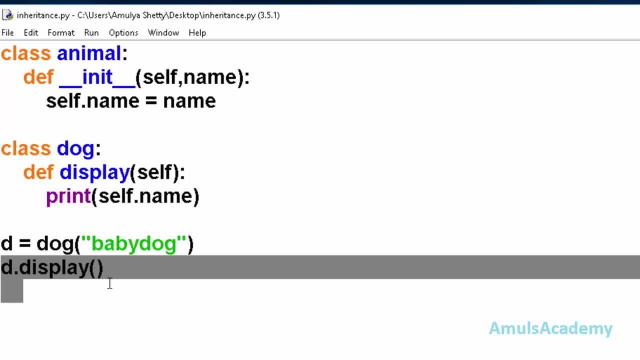 method is public method, so that we can access them outside the class also, But the private methods are not accessible outside the class. Ok, we will see how to define private methods and private variables and how to use this in our program. Ok, Now we will write a program. 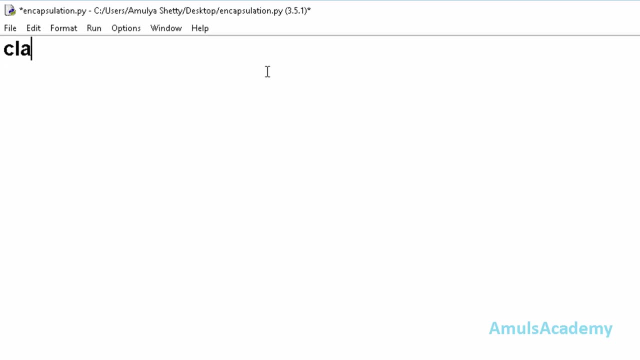 which contains private methods for that class car, and here I will use init method. Now we will use self as the parameter and here self dot. Ok, here this update software is a private method, and here we are calling this method inside the class. Why this is private method. 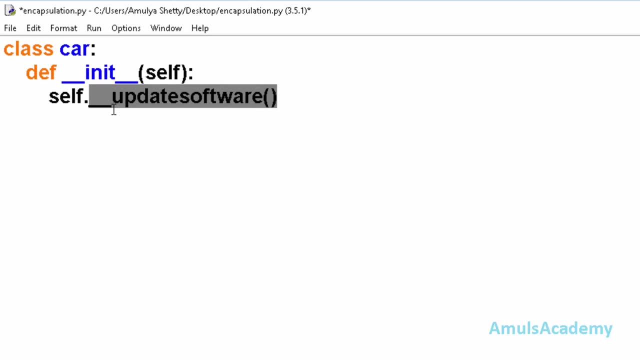 means we can see here two underscores. This indicates that it is a private method. Next I will define another method. It is drive self print- driving. Next. now I will define update software self print. Ok, Now I will go to the private method. Now it is data type. Now, outside the class, I will create: 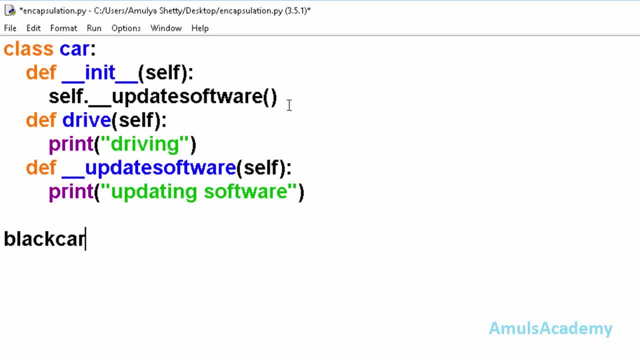 the object black car: ok, car, Now I will call black car. dot drive: Ok, Now I will call my class: Ok, Now I will call my class: Ok. So in this we will define a private model. we will call: I'll save this and run this and here we can see updating software and driving. it's because 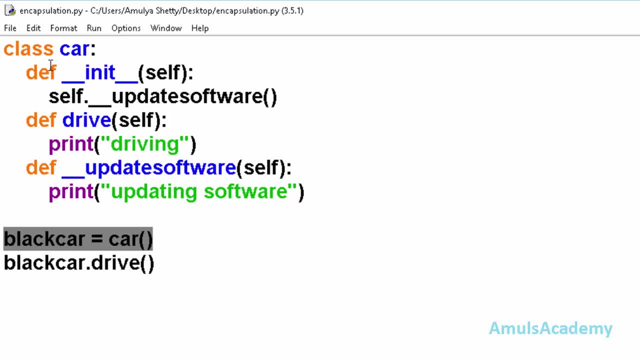 whenever we create object it will automatically call this initialization method. so in this initialization method we called private method, update software, so it will print this message. next we call the drive method, so we are getting driving message here. we can't call this update software outside the class. if we'll do, it will give error. for example, I'll comment this: 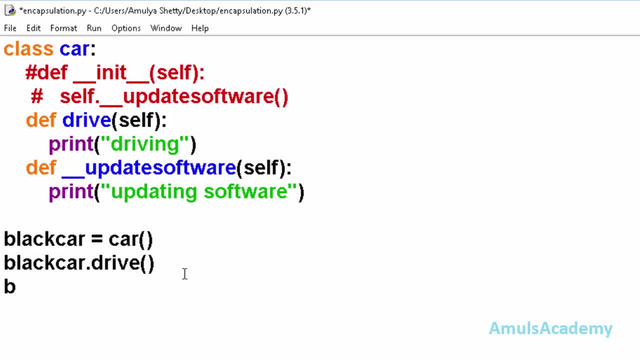 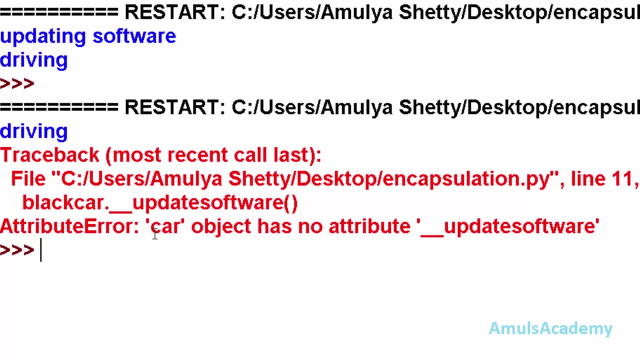 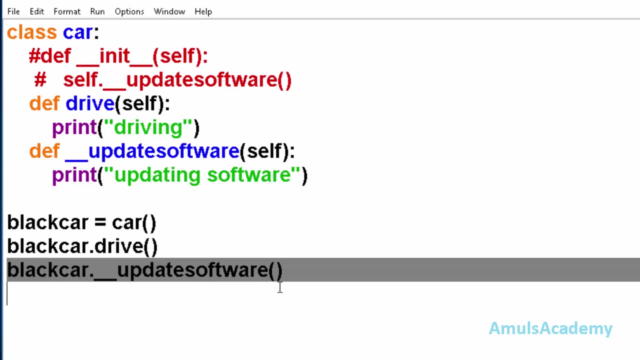 now here: flat car dot. now here we are calling the private method- update software outside the class- and here we are getting error because car object has no attribute: update software. okay, So we can't access this private method outside the class. okay, this is about the private methods. 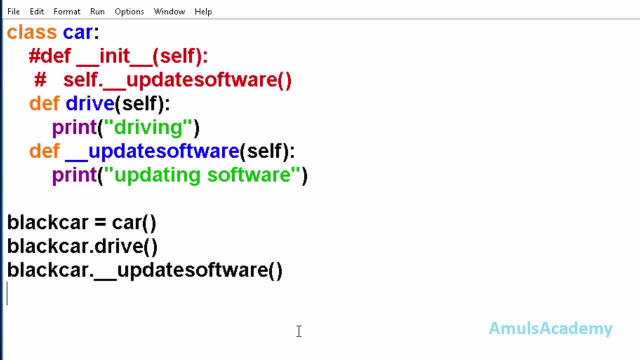 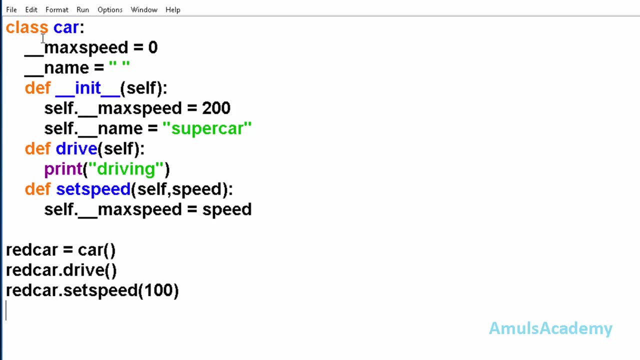 okay, next we'll discuss about the private variables. private variable can modify only inside the class methods. we can't modify private variables outside the class. okay, here we can see an example. this is the class car and here we can see the two variables and beginning of this variable we can see two underscore. that means this is the private variables and we 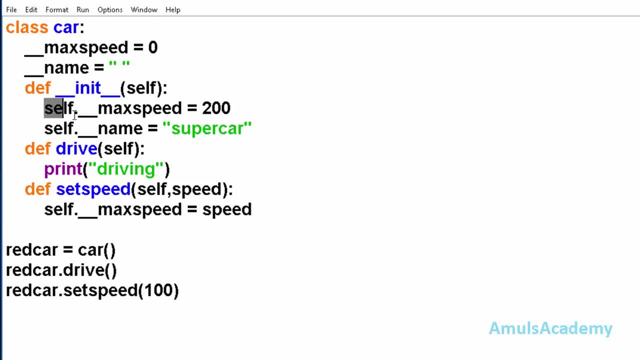 can see the initialization method and here we initialize this: two private variables. next we can see the drive method and set speed method, where we are modifying our private variable. as I said, private variables can be modified inside the class methods and this method is belong to this class. 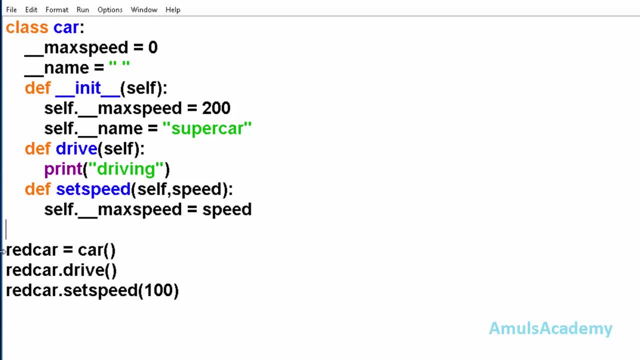 So here we can modify this private variable. Okay, here we created object and we called drive method and set speed method and if you want, we can print this and here we'll print. right now I'll save this and run this and here we can see driving.